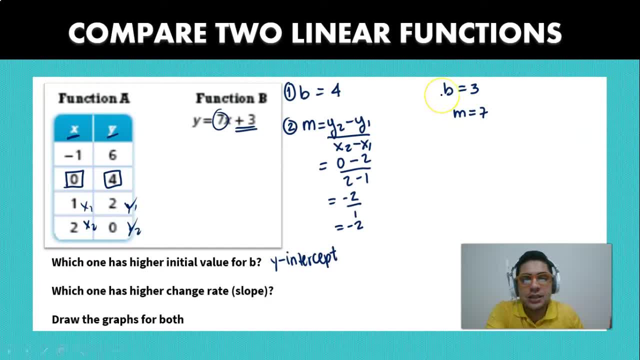 function or the equation. So that means that on the second one- the second one- seven is going to be higher than minus two, and on the first one, four is going to be higher than three. So now they're asking us to write the functions or to draw the graphs. So it's actually. 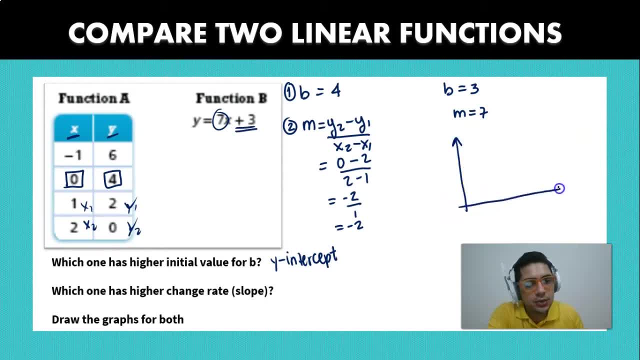 pretty easy. So for function A, we just have to see the points that they give to us. So they give to us point zero, comma, four, Right So zero, one, two, three, four, which we know is going to be our value for the Y intercept, Right So Y and X, and it's going to be four. And 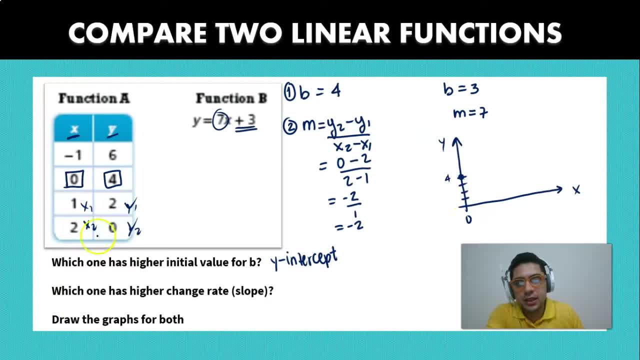 as you can see, for the value of the second value, we can choose this: one, which is zero, and two. So a value of X equal to two gives us a value of zero. So that means that the graph is going to be like this: OK, And this is going to be function. A Right, Now let's 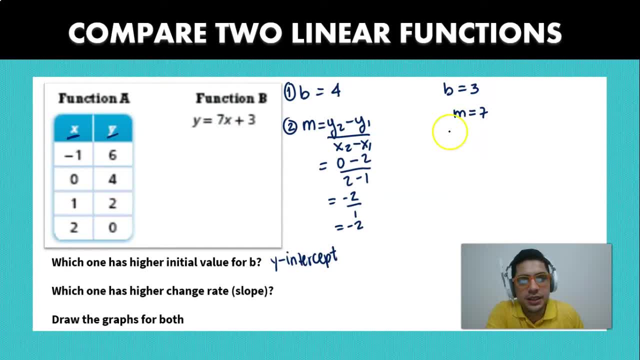 try doing function B. So in the case of our function B we can just graph two points. So we have Y equals seven, X plus three. Let's choose a point. So let's say for X equal to zero. So for X equal to zero, we're going to get the point seven times zero plus three, which 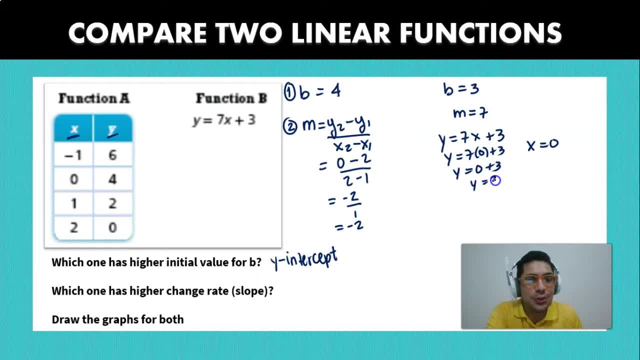 is going to be zero plus three, which is three. So for X equal to zero, our value is going to be Y equal to three. Let's choose a value for Y equals to two, for X equal to two, Right? So it's seven times two plus three. So in this case, it's going to be seven times two. 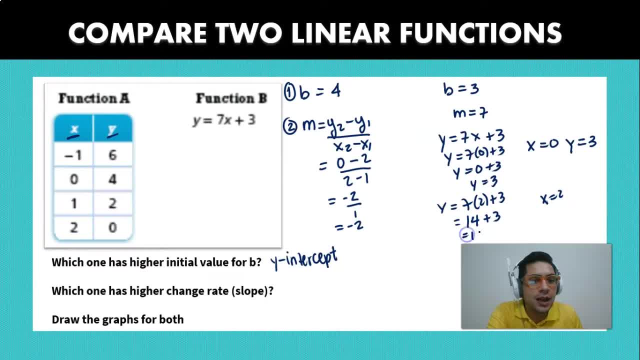 It's going to be fourteen plus three is going to be a value of seventeen. So that means that when X Is equal to two was going to be seventeen. so we can also draw that graph. So it's going to be four, zero. we have a value of one to three and four a value of X. 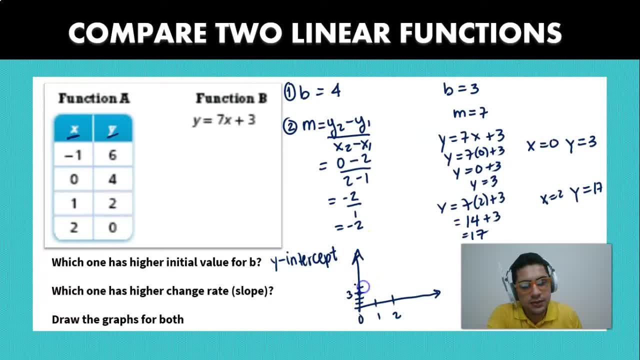 Equal to two. one two, we have a value of seventeen Right, which is going to be around here. I would Just know that it's going to be positive, So it's going to be increasing And it keeps the slope right. so in the first one, since the slope is negative, it goes down, and in the second,